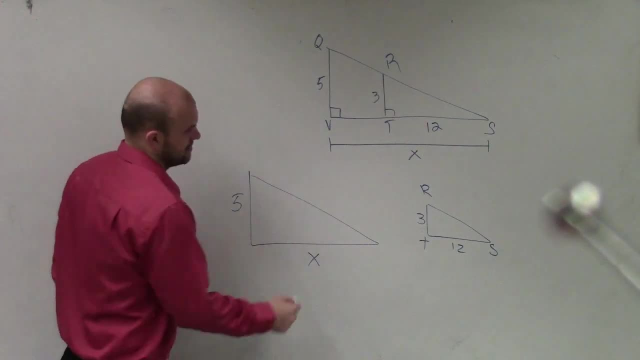 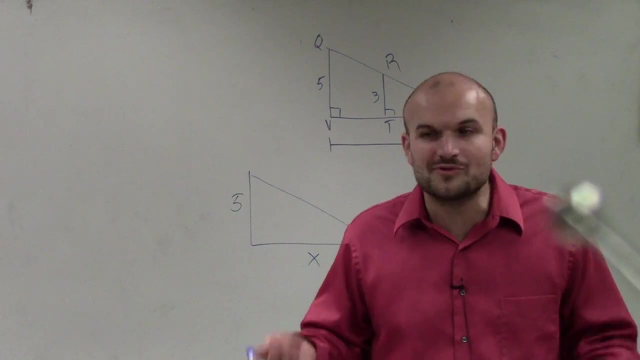 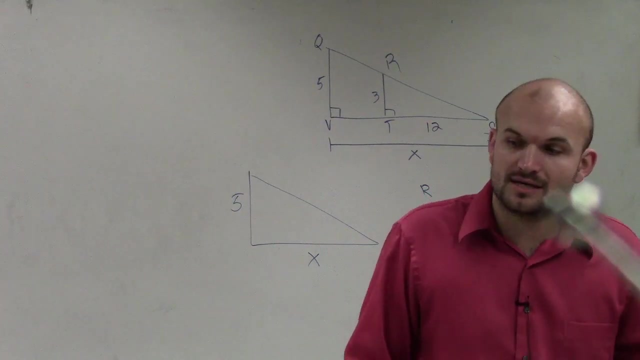 And then they said: this is x, though Right. So to prove similarity, we either need to prove that two of the angles are the same, or we can show that not only are the angles the same, but also that their side lengths are congruent. 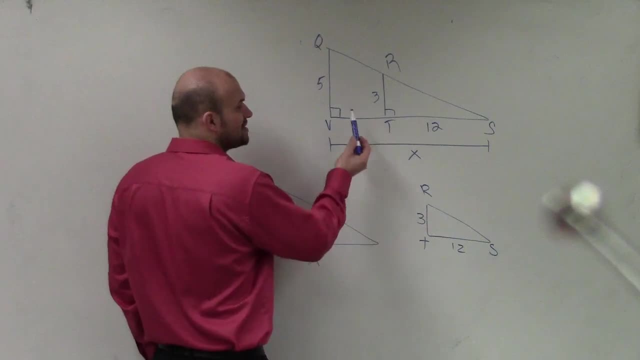 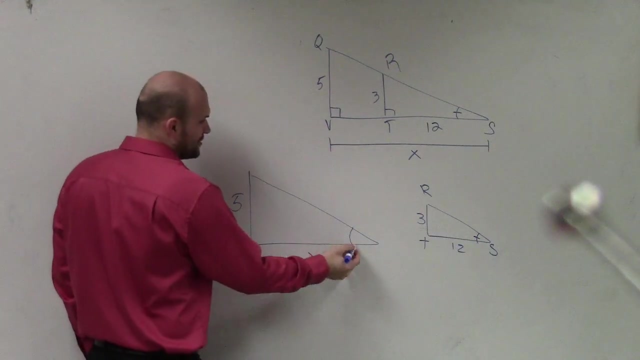 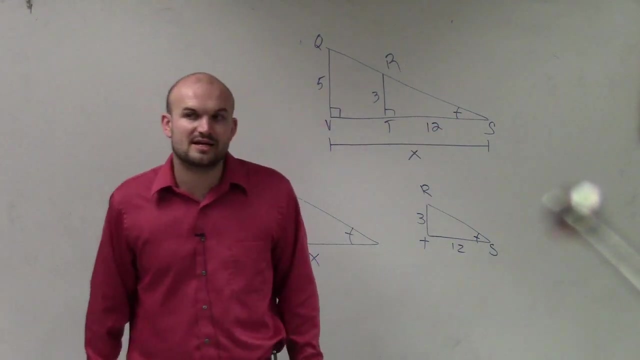 Well, ladies and gentlemen, since these are both right triangles and they share the same angle, can we actually show that these are similar to each other? Yeah, they both already have right angles and they both share the same angle. So I could actually just say right now: 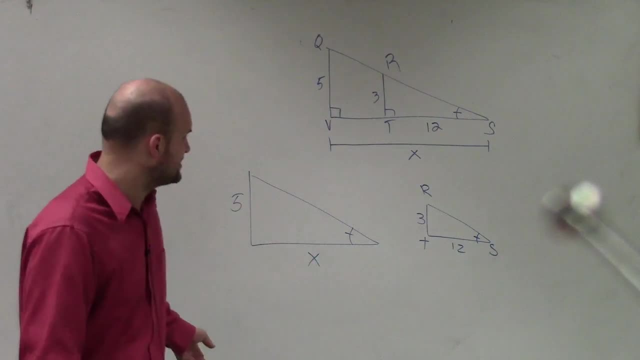 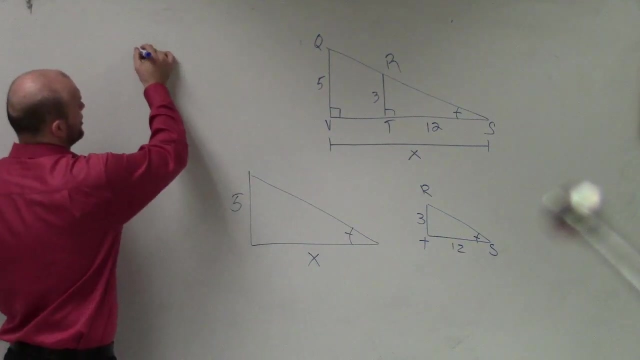 that these are too similar. However, another way to do it would be to say: well, if I can show that these two sides are congruent, and these two sides are congruent. So just to do it this way, real quick, I could always write a proportion, as 3 is to 5, as 12. 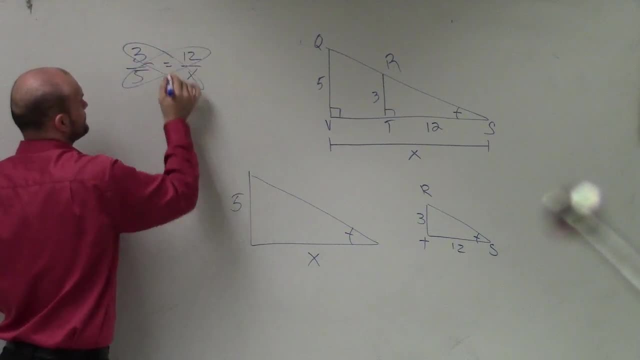 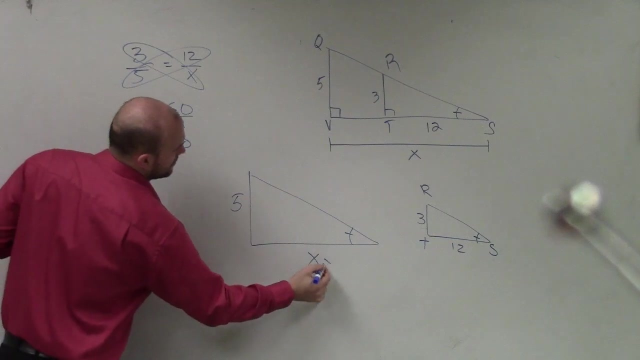 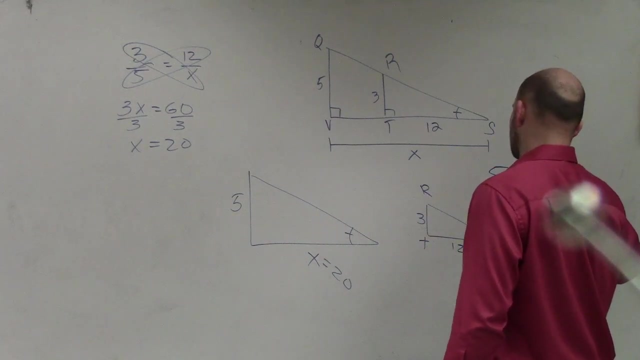 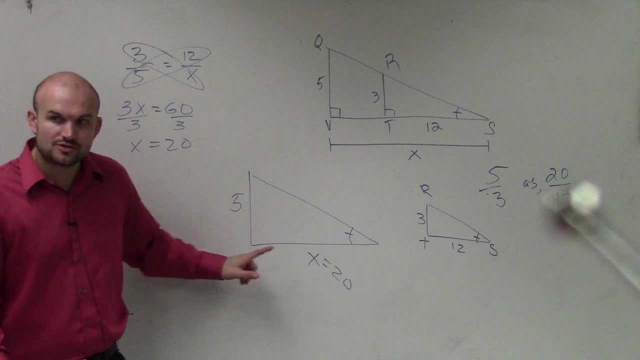 is to x When I cross multiply this way, So 5 is to 20.. So then I'd say: is 5 is to 20, as 5 is to 3, as 20 is to 12?? So what I did, this length is 20.. 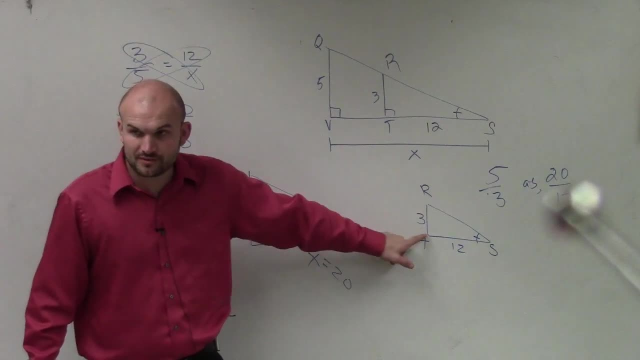 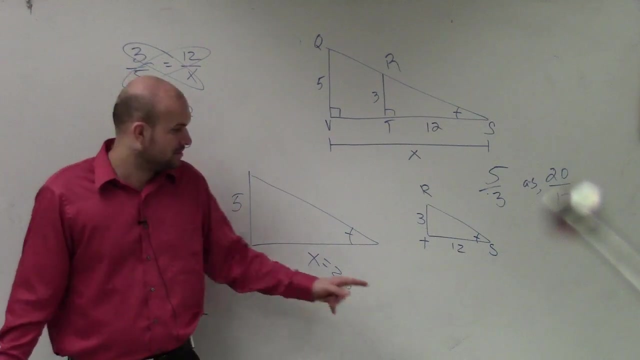 So I wrote a proportion for your side lengths: Is 5 is to 3 as 20?? Is 5 as 20 is to 12? Are those equivalent proportions? Well, where did you get 20 from? I found these two angles x. 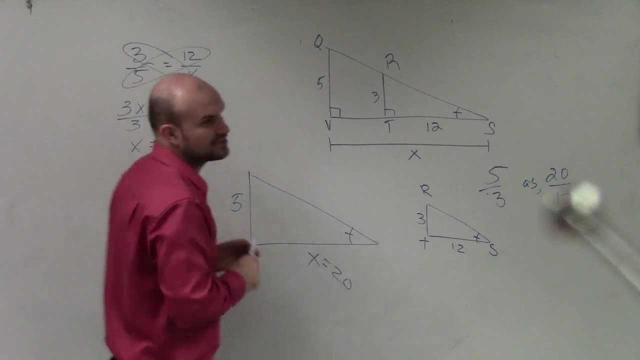 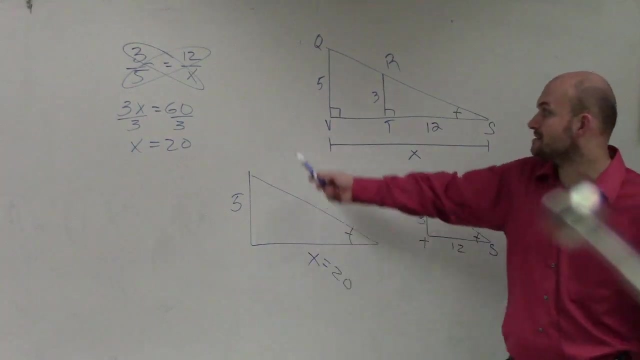 I created a proportion, used cross multiplying and then solved for 20 right here. So I set a proportion as 3 is to 5, as 12 was to x, Set up the proportion cross, multiply and got there. Are these two the same? 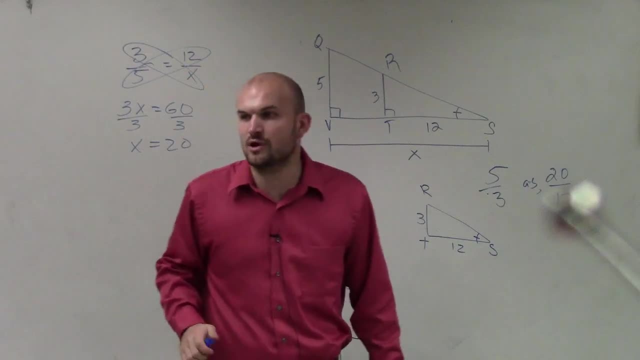 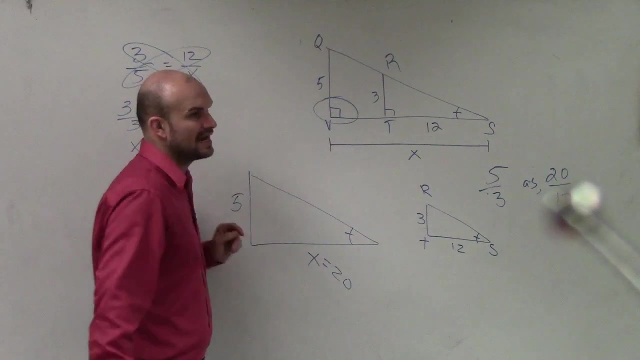 What happens if you divide the top and bottom by 4?? That's 20 over 12.. Then, yeah, it is the same. So you have two proportions for side lengths that are same, as well as an included angle that is the same. 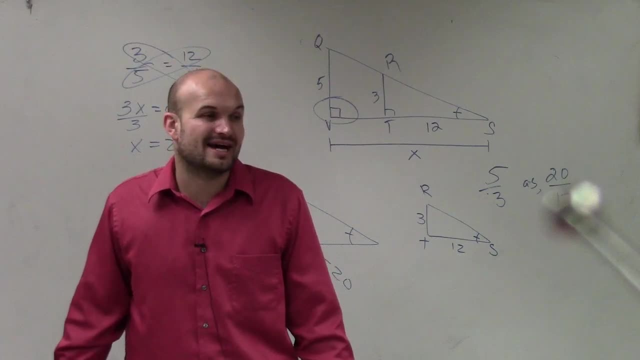 So there's two different ways you guys could say you have similarity: either side, angle side, or by just using angle angle, since they both share an angle.